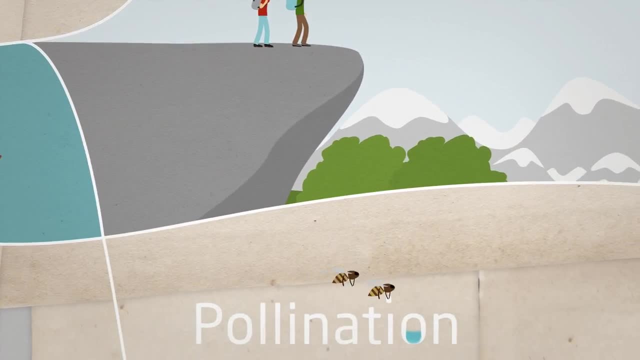 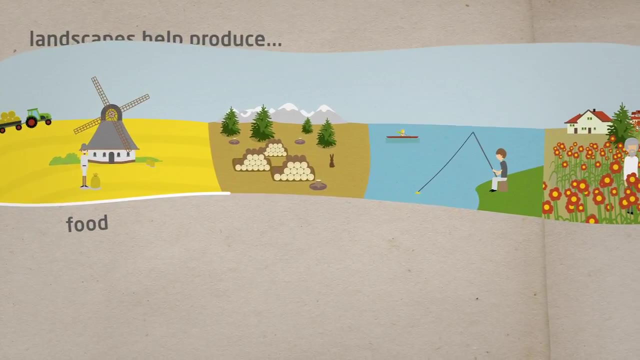 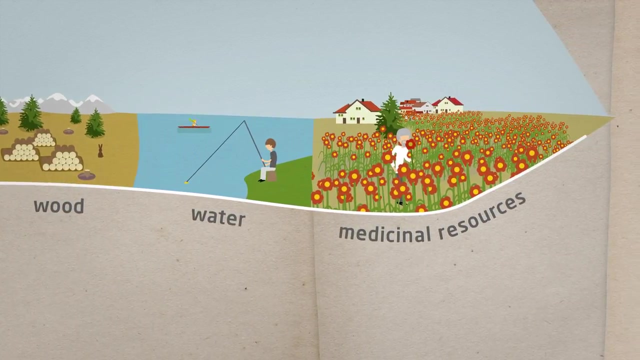 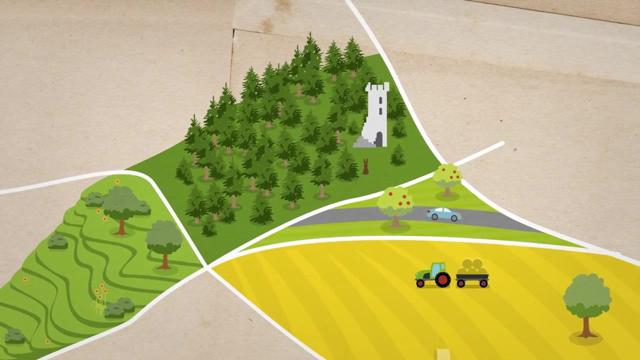 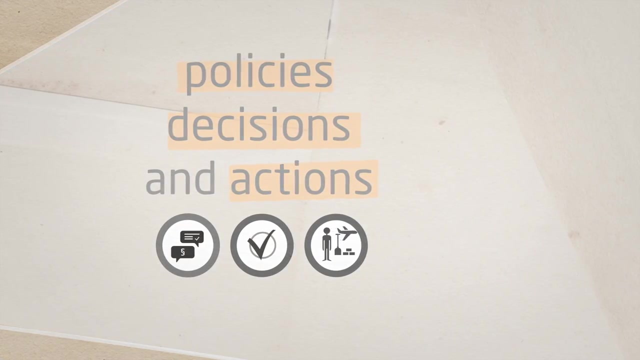 They also regulate services like pollination, water and climate. Finally, landscapes help produce food, raw materials like wood, water or medicinal resources. Our long history has formed our landscapes, their unique appearances and characteristics. Policies, decisions and actions by people living in landscapes, and also by those living far away, can have a profound influence. 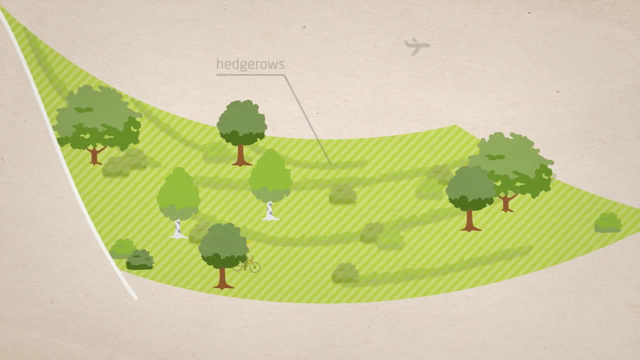 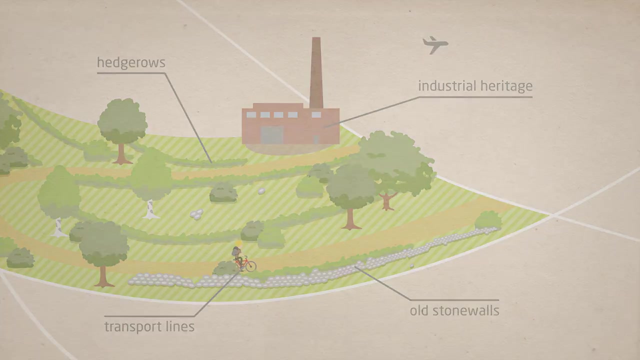 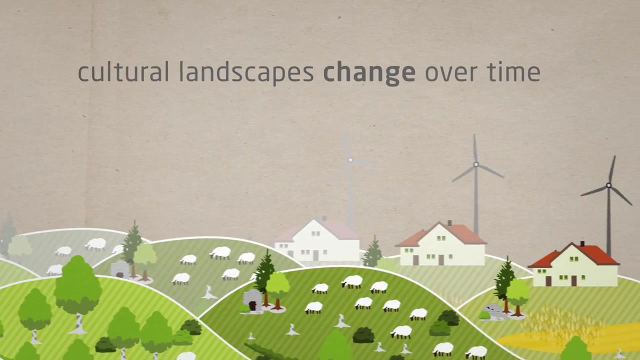 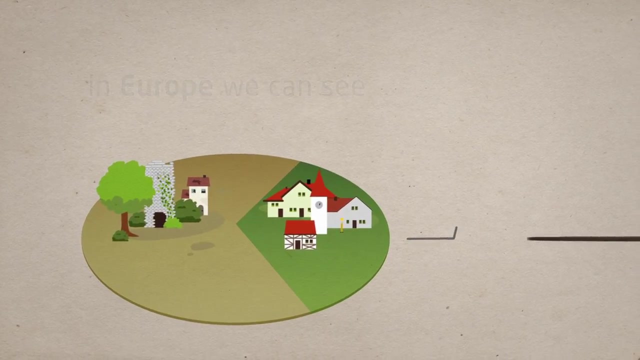 You can see it in hedgerows, transport lines, industrial heritage or old stone walls. Cultural landscapes change over time. However, the modern era has pushed ever faster changes which can threaten their sustainability. In Europe, we can see land abandonment which affects 65% of landscapes. 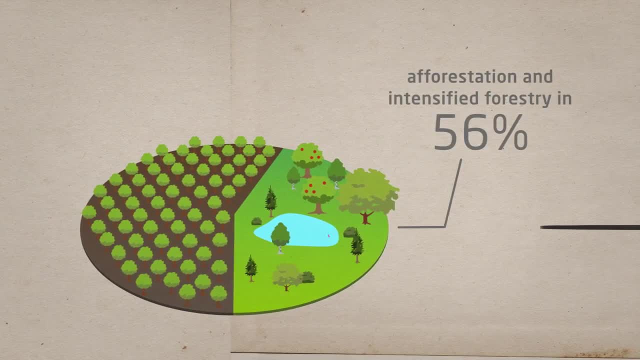 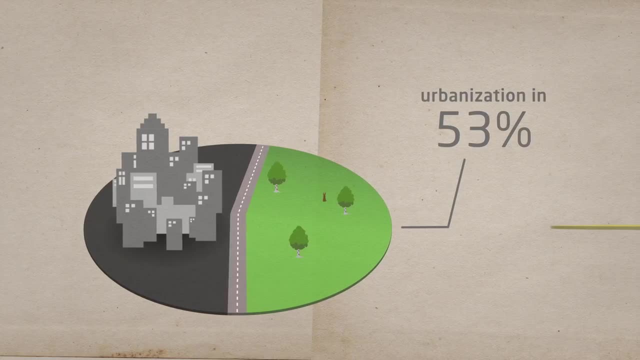 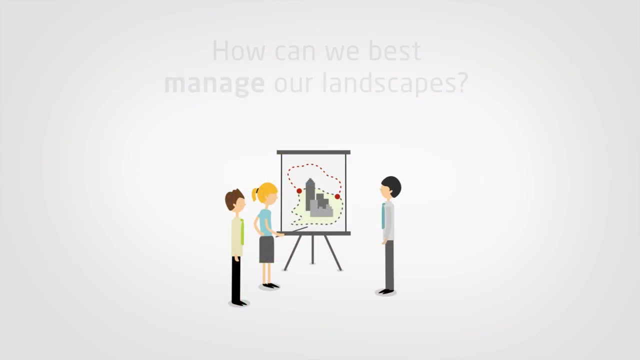 afforestation and intensified forestry in forests. urbanization is an important change process in 53% of landscapes. Agricultural intensification takes place in 62% of landscapes. So how can we best manage our landscapes? A landscape approach means managing multiple land uses in an integrated manner. 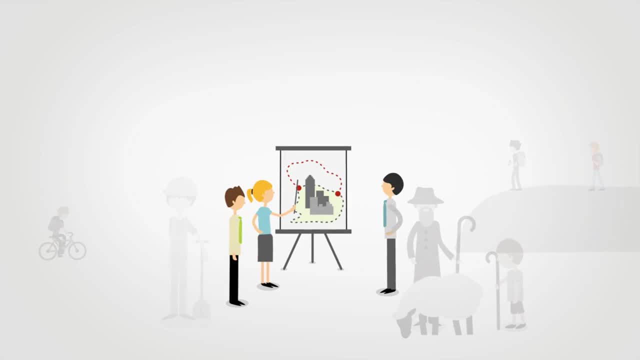 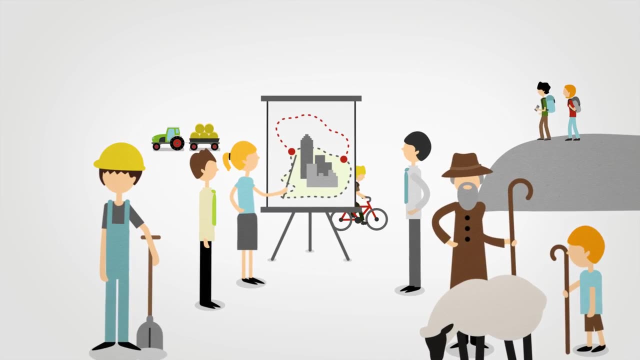 It considers the environment and human processes that help shape our land, as well as the environmental impact of the environment. It also considers the environmental impact of the environment and human processes that can help shape our land, as well as the health and happiness we get from it. 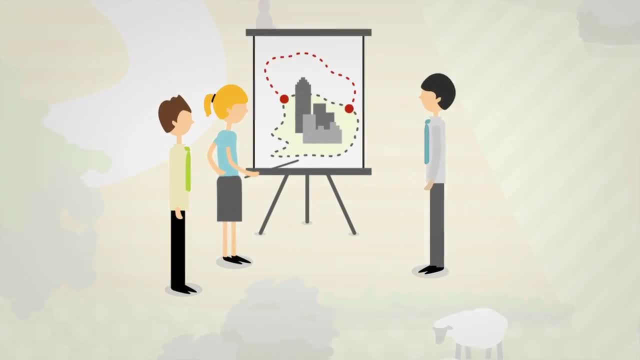 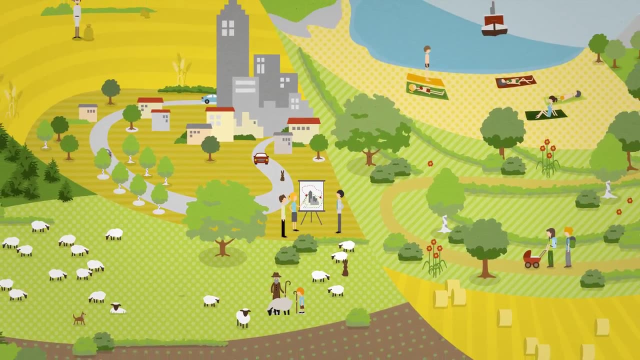 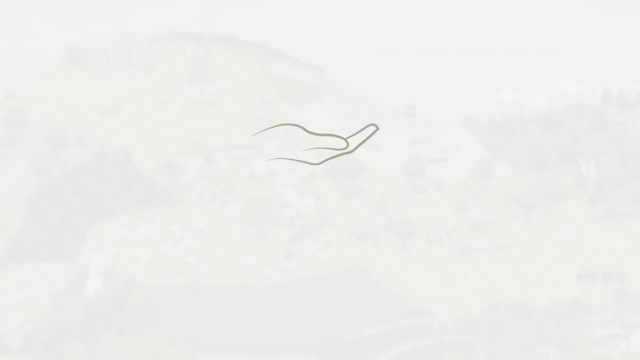 European landscapes are dynamic. To cherish them and provide a future, we must see the whole picture. All its uses belong together. For more information, visit wwweuropeorg.